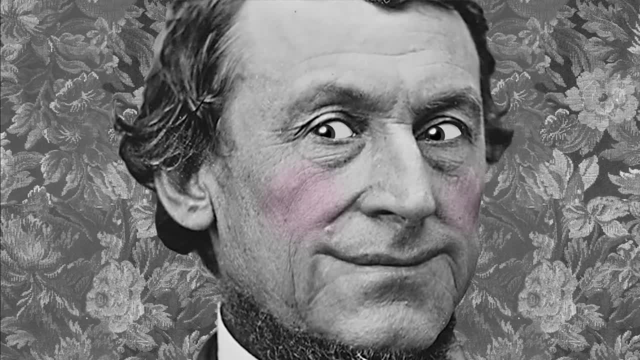 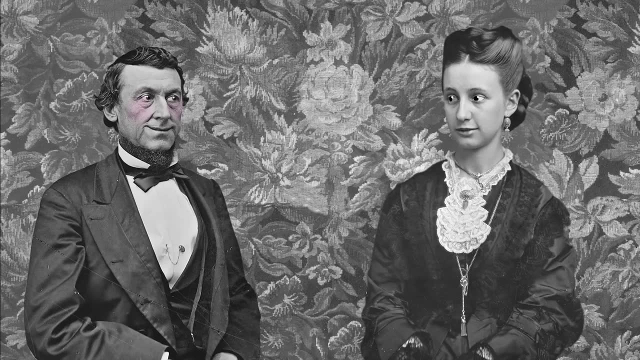 Darcy's eyes linger on Lizzie's face and how he seems all flustered when she's around. Add to the mix your knowledge that Mr Darcy is in a much higher social class than Lizzie, and your sense of insight should be telling you that there's something more here In this. 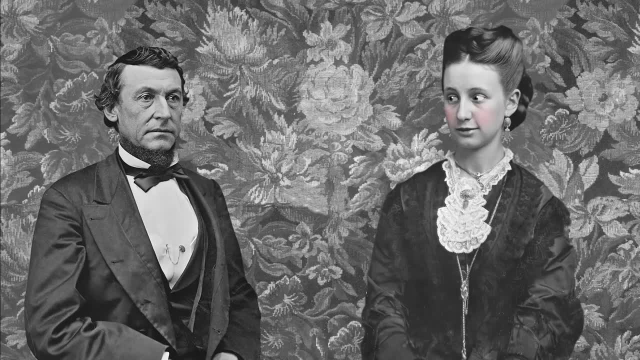 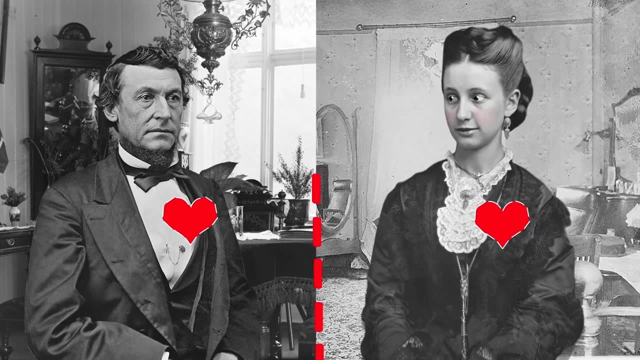 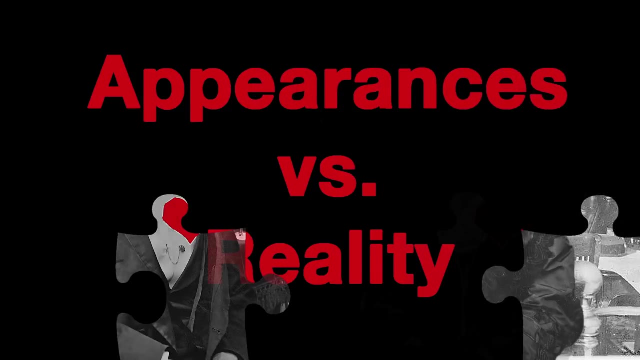 case, it will tell you that Darcy's surface behavior is incomprehensible. Think about all those small clues. gives us insight about some of the big abstract ideas within the novel that we can approach in an essay. Appearances versus reality, the power. 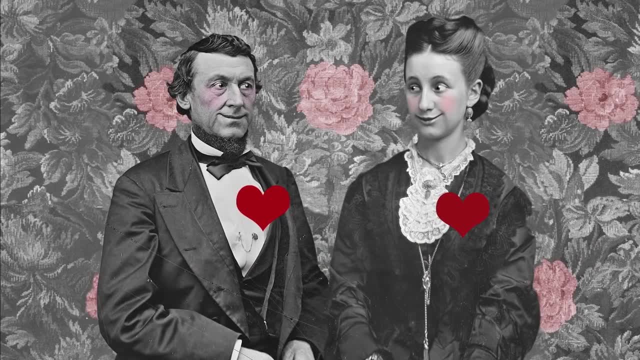 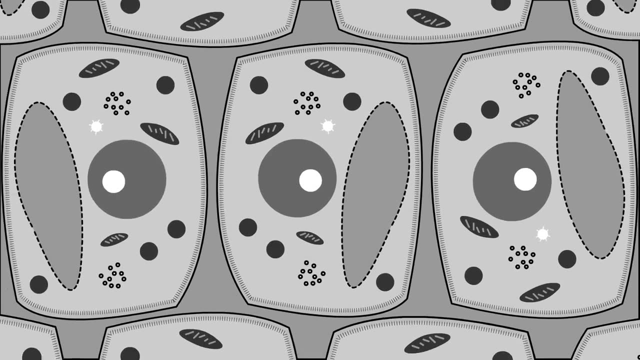 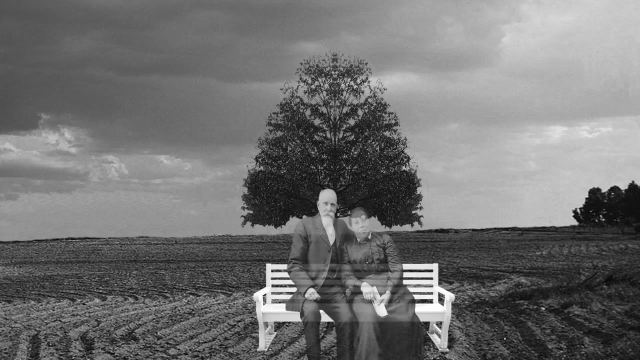 of wealth and social stratification and the unpredictable nature of love and attraction. Look at that Deeper meaning. The second step to a sophisticated analysis is acknowledging complexity. Let's face it: Both life and literature situations are complicated due to social forces like relationships, moral. 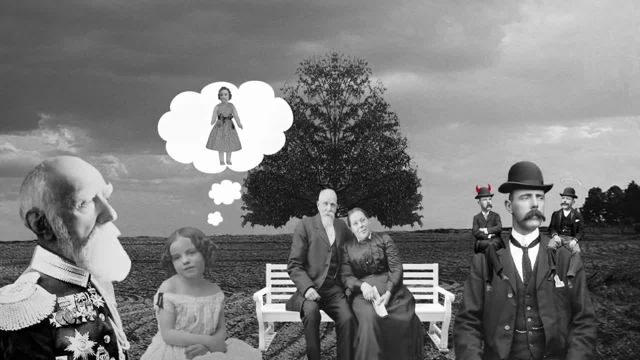 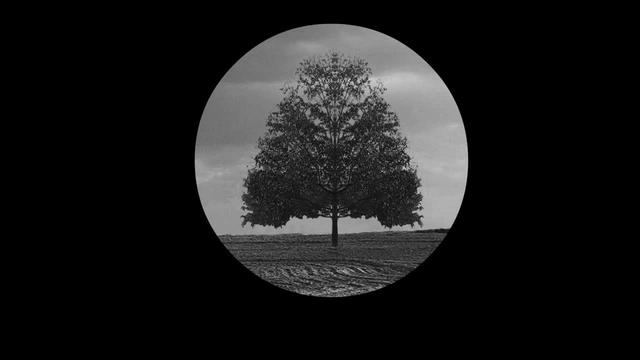 codes, personal desires and power structures. This means that there are, at any given time, multiple factors that shape what is true. In order to acknowledge complexity in your writing, refrain from making broad generalizations about a text or establishing quick, simple judgments about a character. 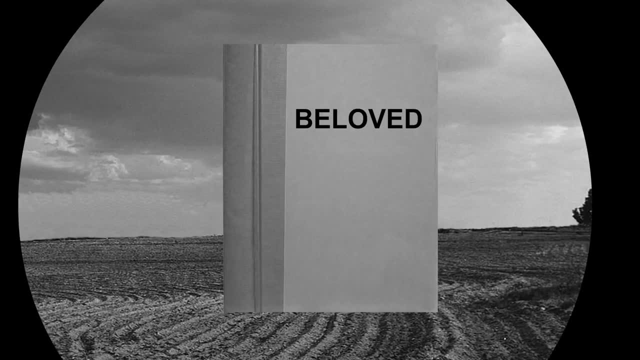 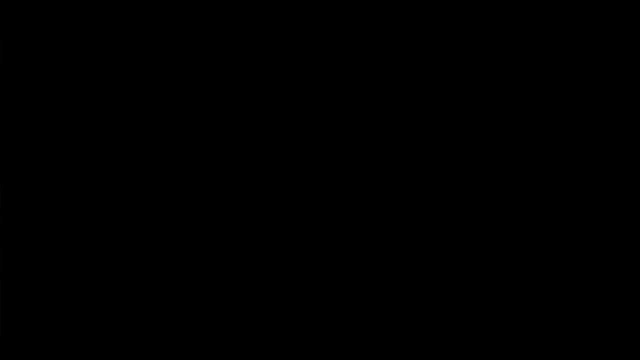 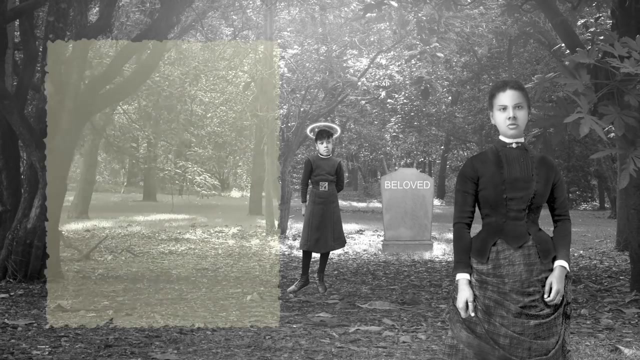 Explore each facet of your subject carefully and make sure to consider multiple influences on events. Explain the tension of multiple forces that create the story. For example, a basic analysis of Toni Morrison's Beloved, where the protagonist has killed her own child rather than allow her to grow up in slavery, might sound like this. 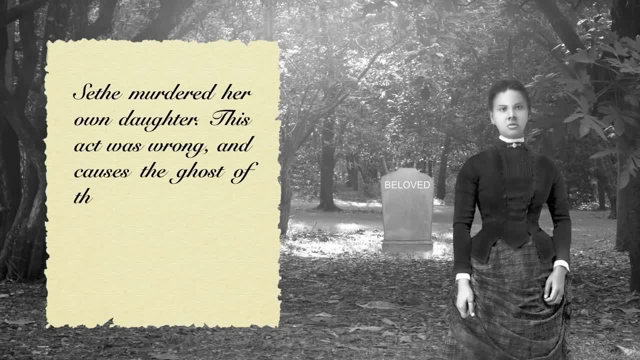 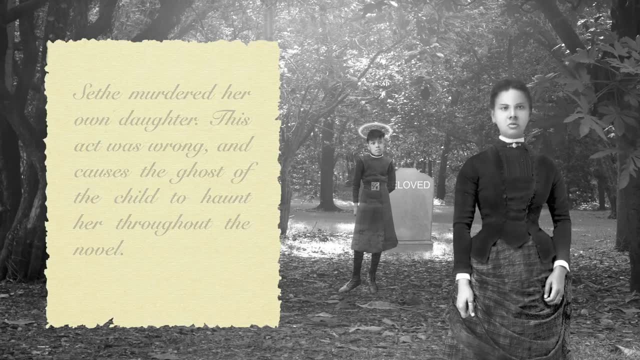 Sethe murdered her own daughter. This act was wrong and causes the ghost of the child to haunt her throughout the novel. These observations are simplistic. They don't acknowledge all the different forces that contribute to what the character has done. Try something like this instead. 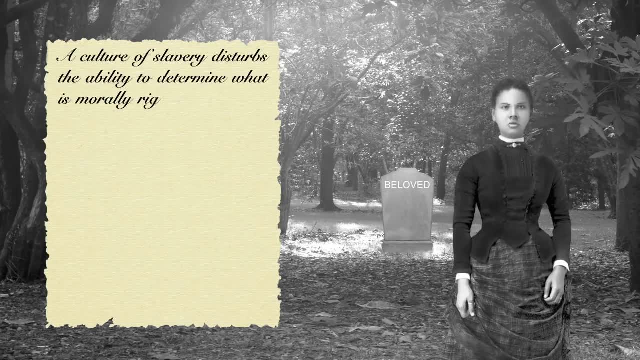 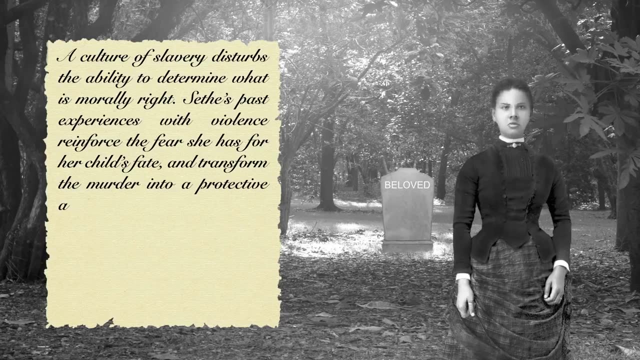 A culture of slavery disturbs the individual. Sethe's past experiences with violence reinforce the fear she has for her child's fate and transform the murder into a protective act. As the novel progresses, Sethe is haunted both by the angry spirit of her daughter and 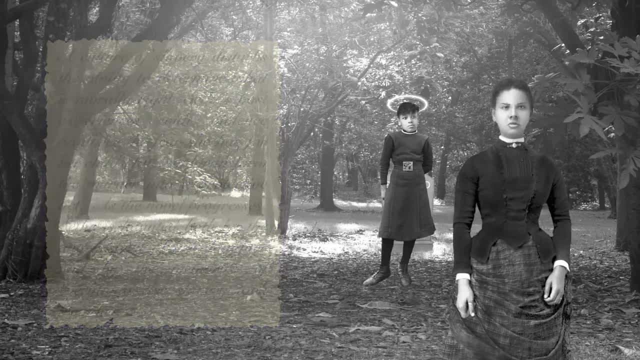 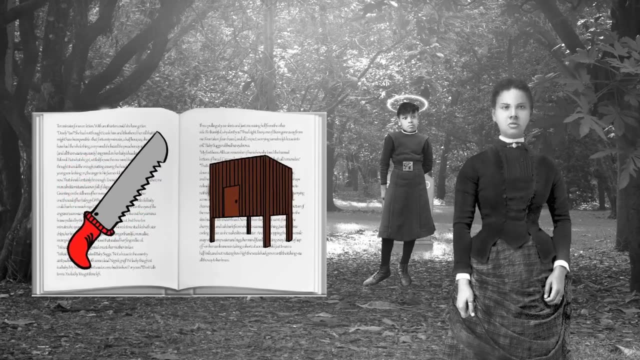 by the memories of everything else slavery took from her. Here we see those influential forces at work and we've shown off our ability to understand the complicated nature of the human experience, which again allows us to access those big ideas that reveal the deeper meaning of a story.